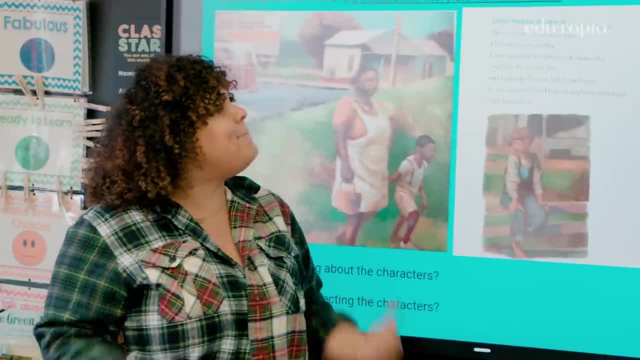 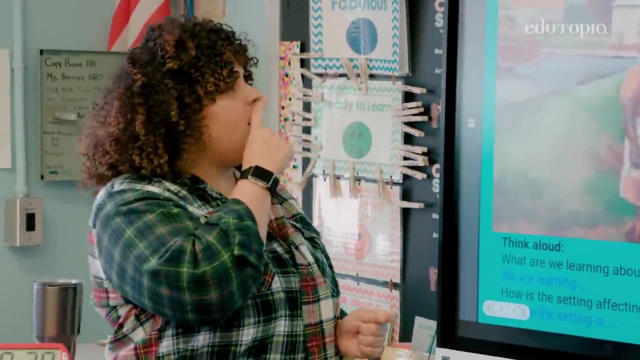 All right, let's start with our first page. John Henry Waddell is my best friend. His mama works for my mama. Wait a minute. I feel like that narrator is inside the story, so it must be first person Even on the first page. I want to do that. Think Aloud work that the majority of the 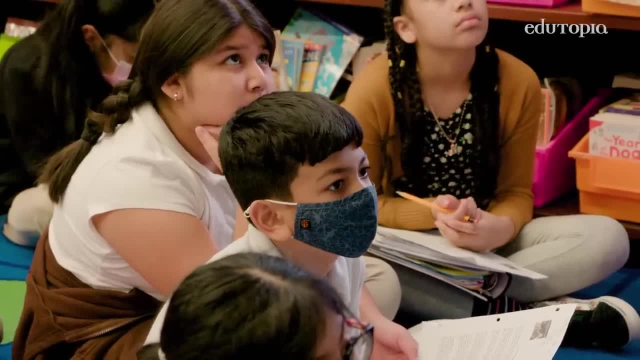 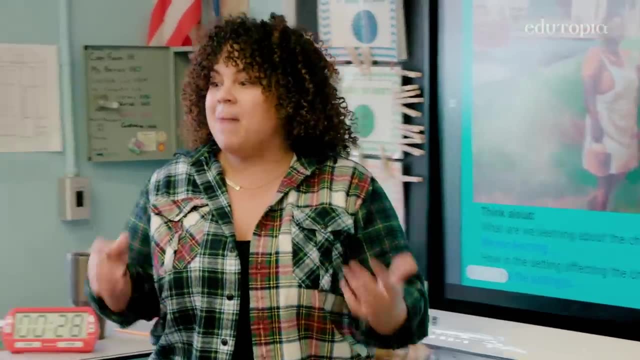 room is not going to do on their own. What are those deeper ideas we're seeing here? Why is the setting so important? I feel like the fact that John Henry's mother works for Joe's mother might cause some big problems in their friendship. 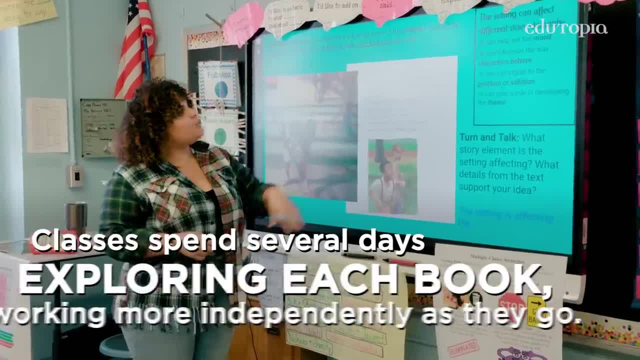 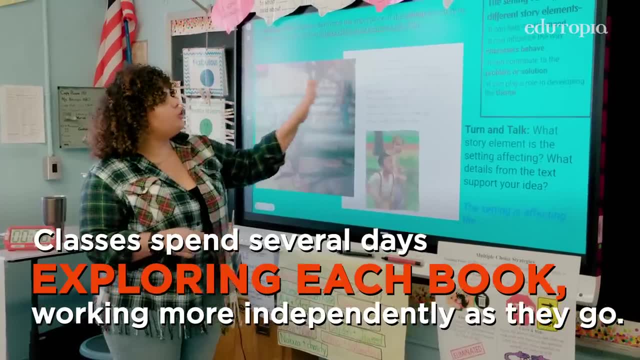 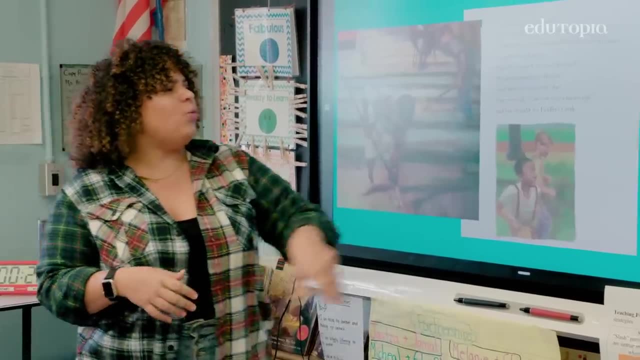 So let's move on to the next page. We shell butter beans, We sweep the front porch. Whatever your teaching point is for that, read aloud. that's when you want to stop and do this work. It won't be every page. You want to be strategic? Then we run straight for Fiddler's Creek. So I want to think to myself. 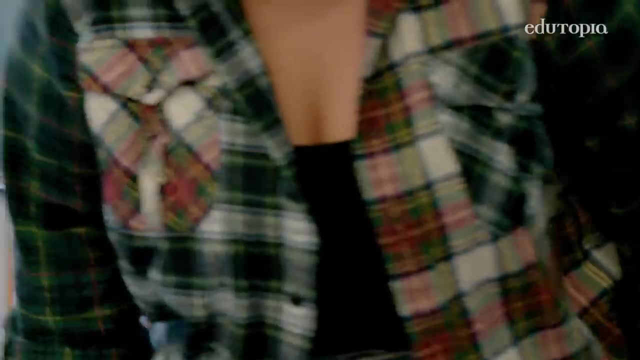 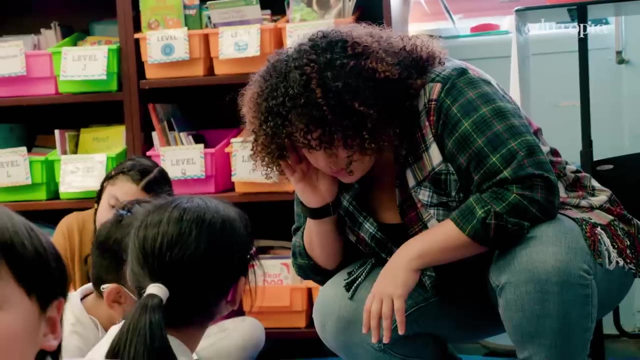 what story element is the setting affecting here? You're going to turn and talk to your partner. Even though they are different, they still find their own solution to spend time together. I get to listen in to all these turn and talks and get an informal assessment of what kids are. 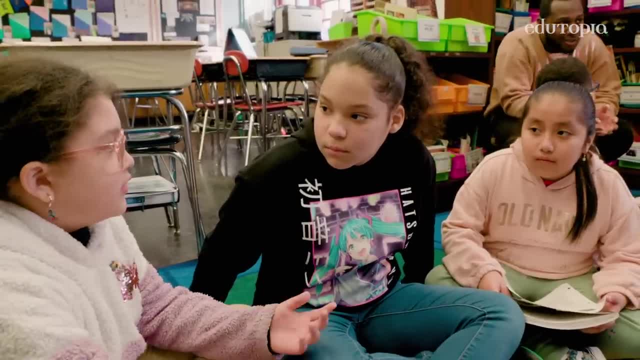 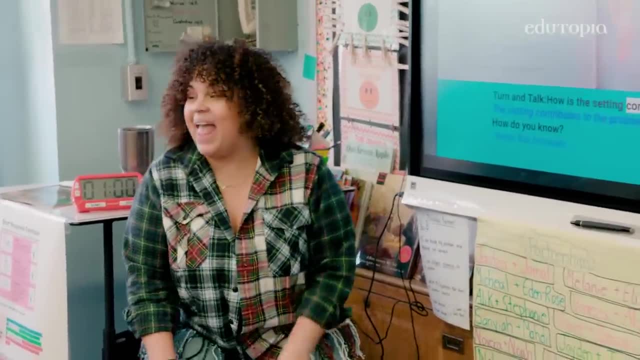 thinking about these texts. How are they responding to this question? All right, let's come back together. I heard some of my partnerships talking that the setting is contributing to the problem and the solution because, although they can't play at the town pool, do they have a cool? 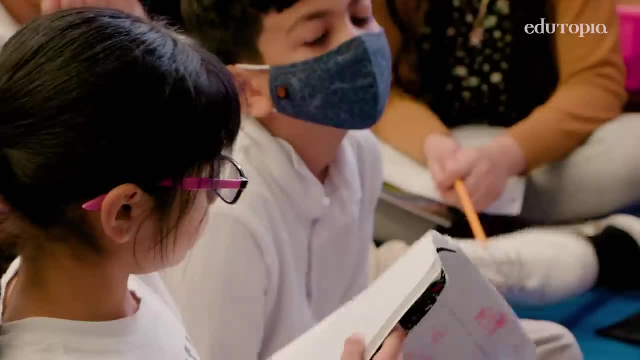 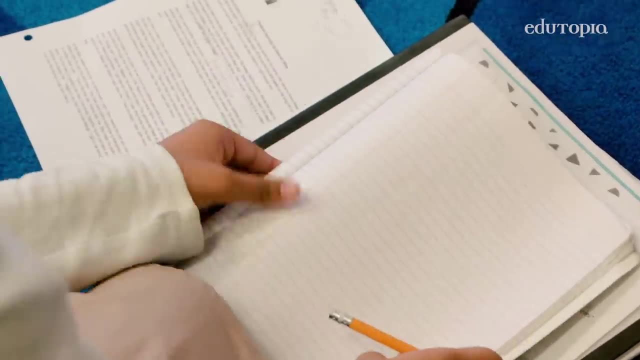 creek to go play in, Totally. So I want you guys to open up your notebooks and we're going to answer the question: How is the setting important to the story? You can say the setting is important because it affects, develops, creates, shows, 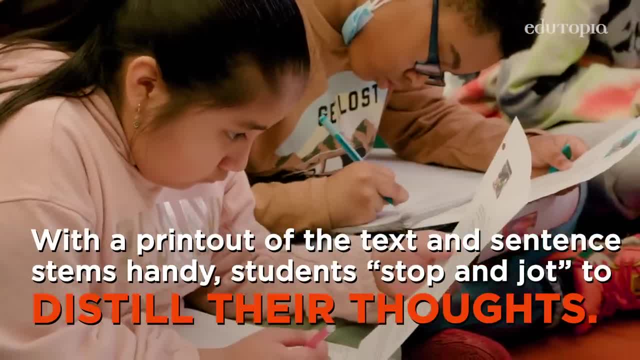 Right. So the setting is important because it affects, develops, creates shows. Right. So the setting is important because it affects, develops, creates shows. The stop and jots are to do that final thinking work. The setting was really important in this book. 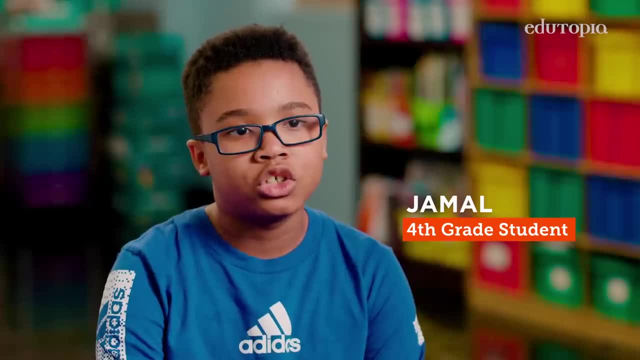 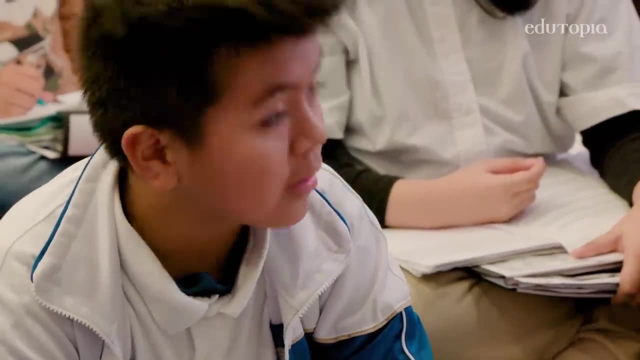 because the white kid and the black kid couldn't do as much stuff together. During 1960, people of color were not allowed to pull the ice cream shops or any other places, So Joe finds alternative ways to help. I want the kids to see reading can be fun.